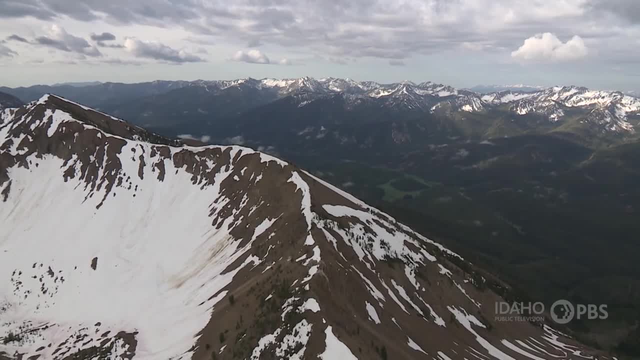 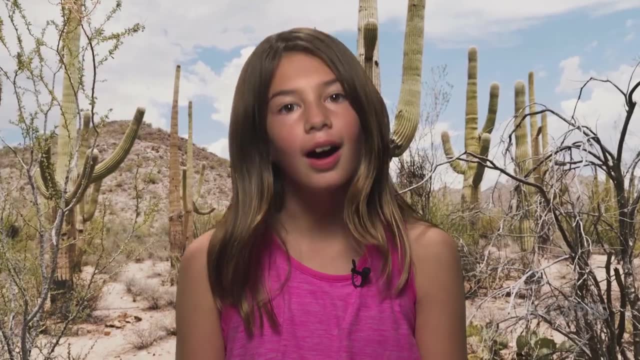 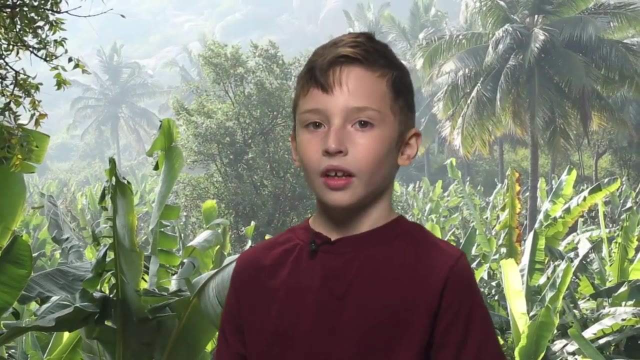 Weather patterns describe a climate, and climates generally have the same weather patterns year in and year out. Man, it's cold, It's hot, It's a little chilly, It's not bad, It's humid. The earth is divided into five basic types of climates, and those can be broken down into: 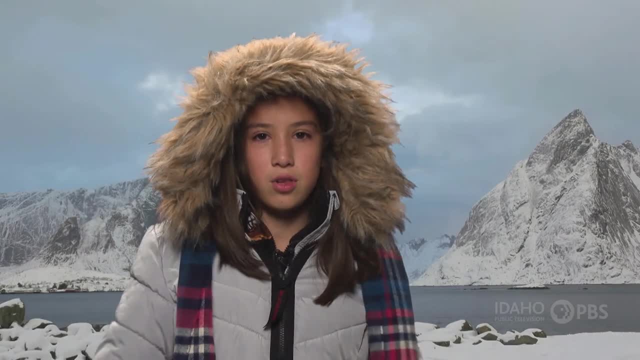 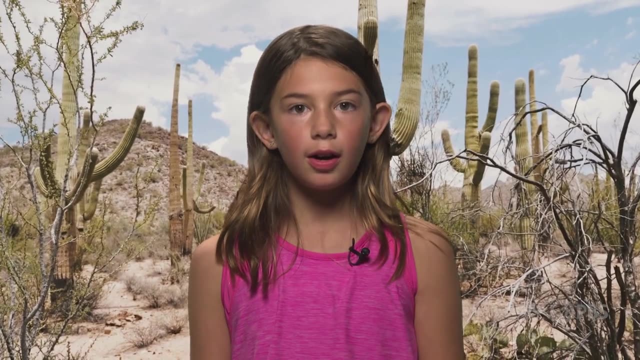 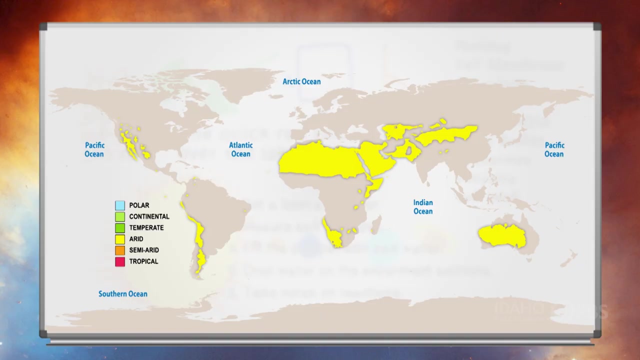 subcategories. Polar climates are cold and dry, with long winters and short summers. The Arctic region is a polar climate. Dry climates have hot days and little rainfall. Arid climates are found in the southwest United States, North Africa and much of Australia. Semi-arid climates: 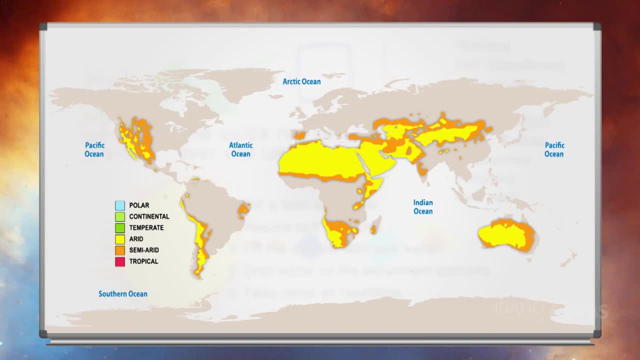 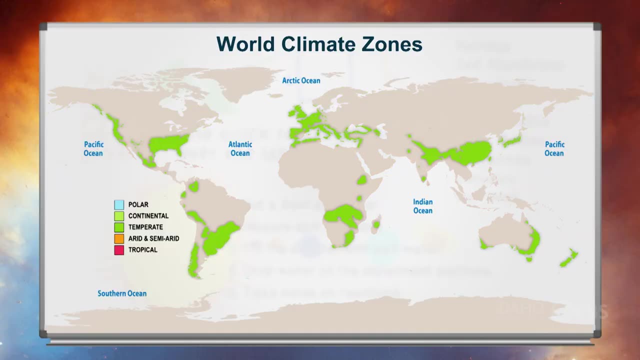 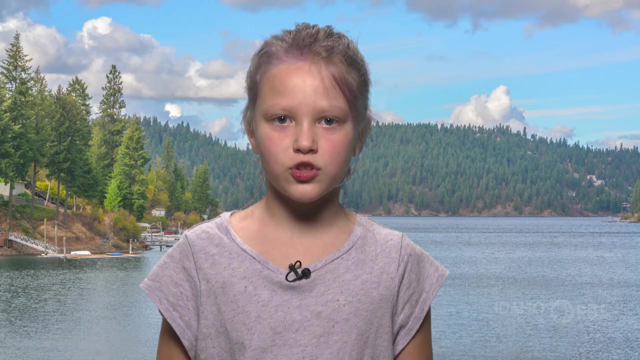 are found in Central Asia and the Great Basin states in America, including southern Idaho. Temperate or moderate climates have warm summers and mild winters, like along the eastern United States and the Pacific Northwest. Continental climates have cold, snowy winters and cool summers. You'll find this climate in 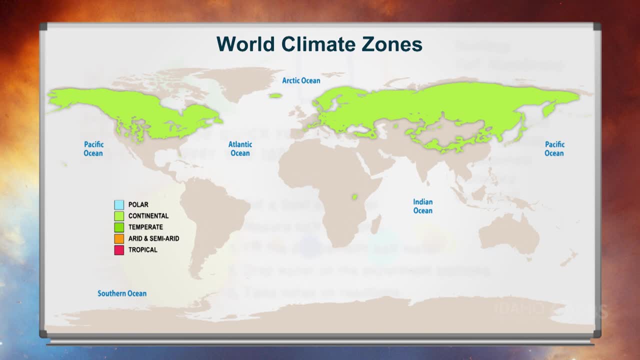 much of Europe and the northern United States, including north Idaho. Tropical climates are found in parts of South America, India, Africa and Indonesia. The climate is hot, humid, with lots of rain and warm temperatures year round. So why does the earth have so many different? 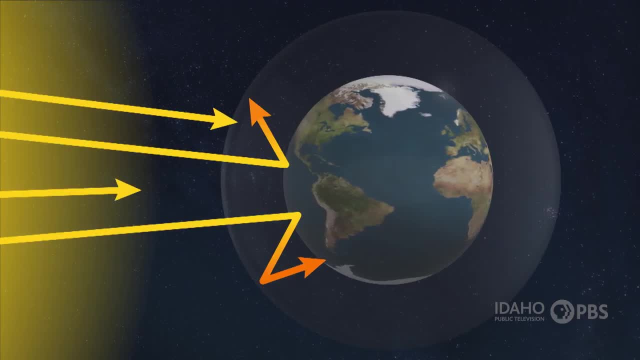 types of climates? Well, it's because of the different ways the sun's energy moves in and out of the atmosphere and how that energy moves around the planet. And lots of things can influence the sun's energy as it spreads around the world. One is latitude The earth has. 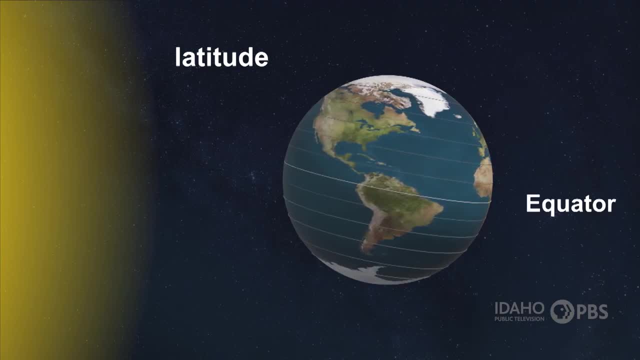 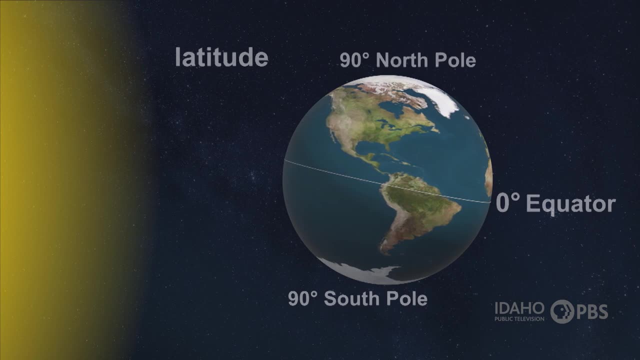 a line going around its center called the equator, and there are other parallel lines dividing up the planet north and south. Latitude marks where you are between the equator and one of the poles and how much sunlight an area gets helps determine that latitude's climate. 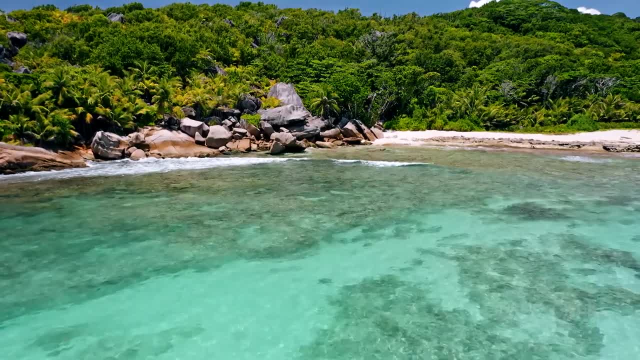 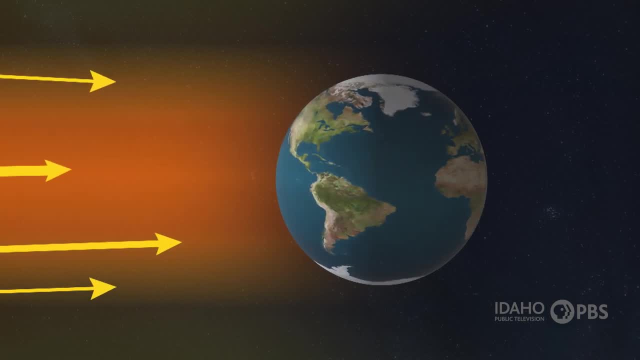 Because the equator gets the most direct sunlight, temperatures there are warmer. But as the sun's energy angles over the curvature of the earth, it doesn't hit as directly, so areas receiving less sunlight have lower temperatures. And because the earth tilts, it can't hit as directly, so areas receiving less sunlight have lower temperatures. 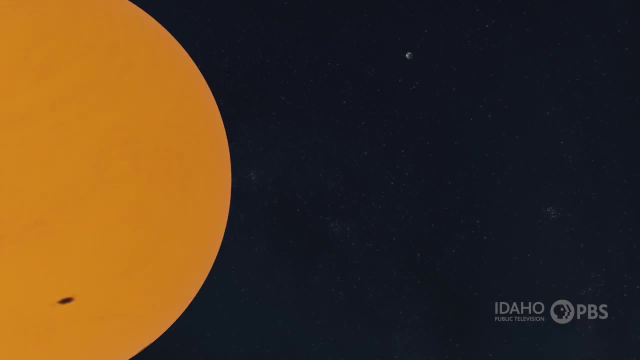 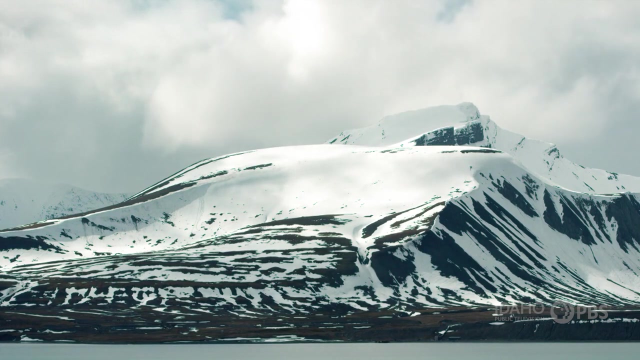 on its axis. either north or the south pole is pointed away from the Sun, depending on where the Earth is in its yearly orbit. When a pole is tilted away from the Sun, it gets less sunlight, so it has colder temperatures. Other things can. 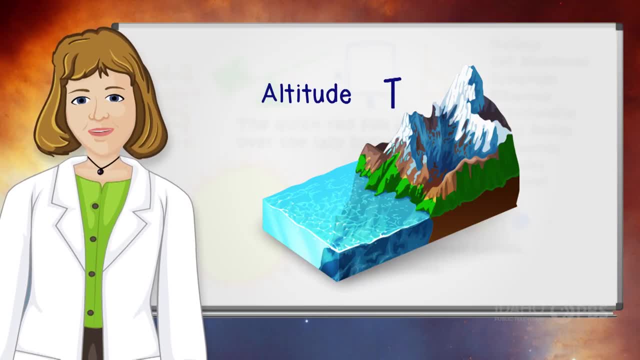 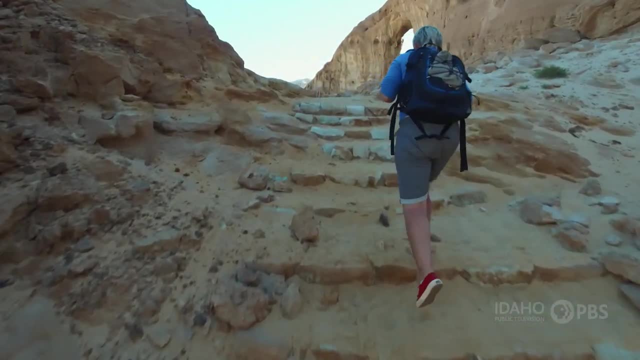 affect an area's climate. Altitude is one way we measure the distance from where you are to sea level. When you go up into the mountains or up in altitude, the air is less or thinner. That's because gravity pulls air closer to the Earth's surface. 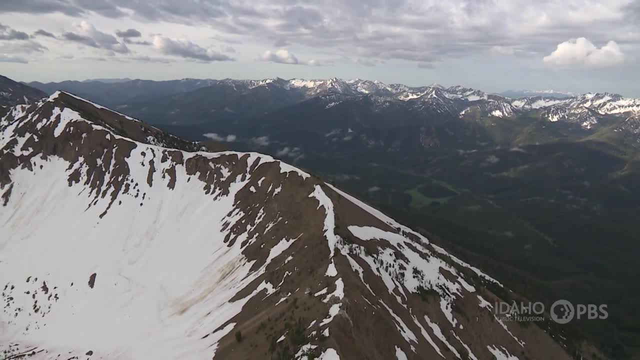 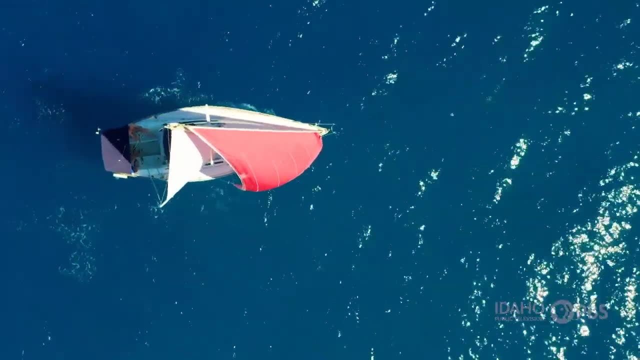 Thinner air is less able to absorb and store heat from the Sun, so the higher the altitude, the cooler the temperatures. Having a large body of water nearby can also influence what kind of climate an area has. Water absorbs and stores heat, So if you live near the ocean, your climate tends to be. 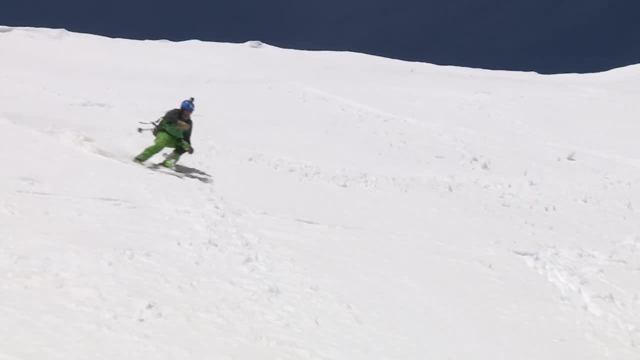 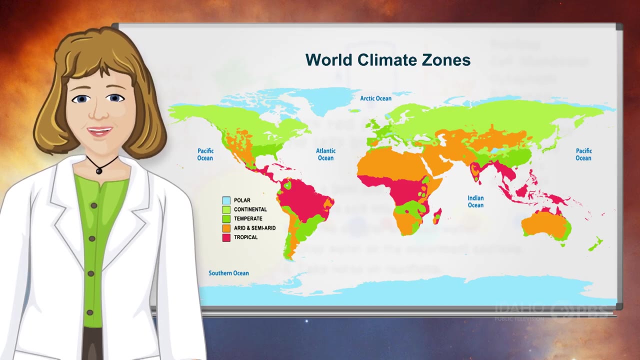 milder wetter and have less variation, Live far away from the ocean or a very large lake, and your high and low temperatures tend to be more extreme. So the regional climate in your area depends upon where you are on Earth, what your elevation is and what geological features like lakes and 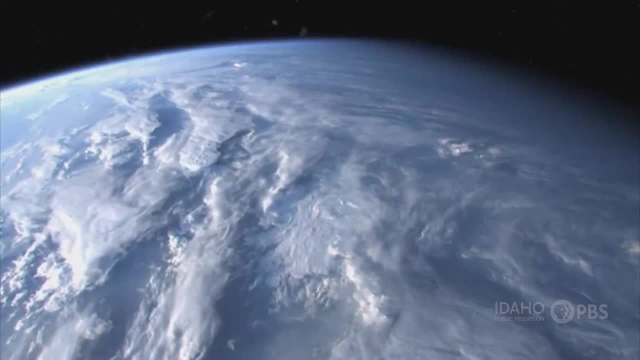 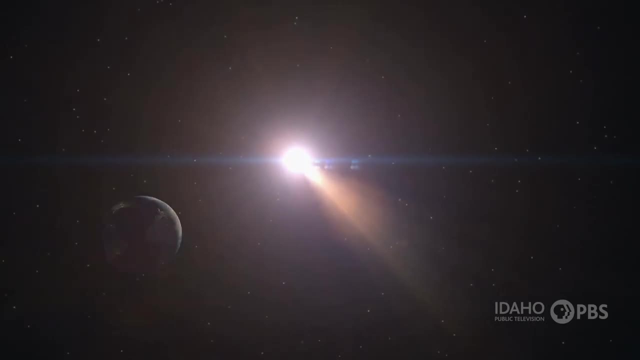 mountains are nearby, But there's also a global climate. The global climate describes the condition of the planet as a whole. It has a lot to do with how much energy the Earth receives from the Sun and the amount of energy trapped inside the atmosphere. Earth's climate has changed many times over the eons. Usually, 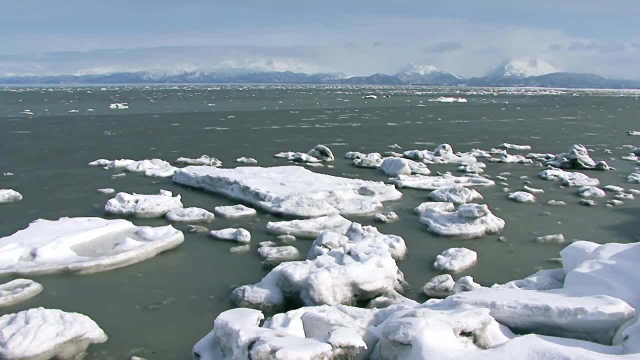 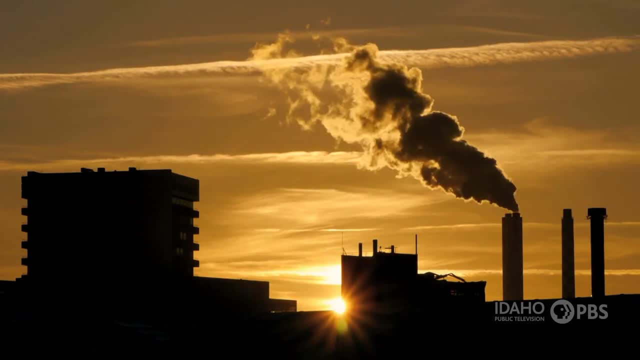 it takes thousands of years for a global climate to change, But scientists report that the Earth is now warming faster than it ever has in the past, and research shows it's mostly because of human activities. When we burn fossil fuels like oil, coal and gas, carbon dioxide is released. The buildup of 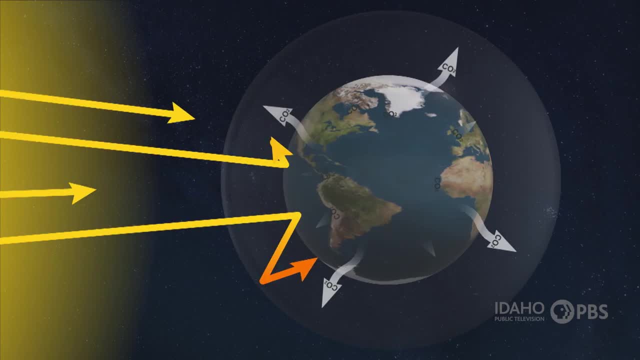 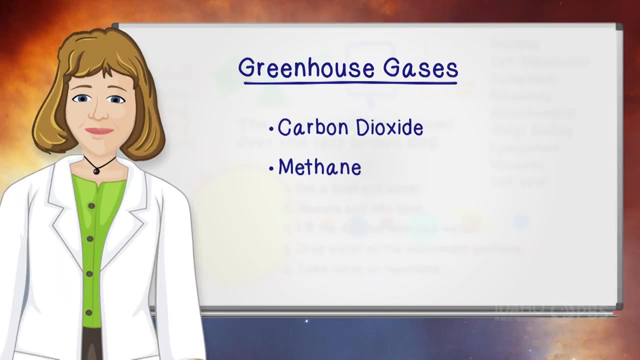 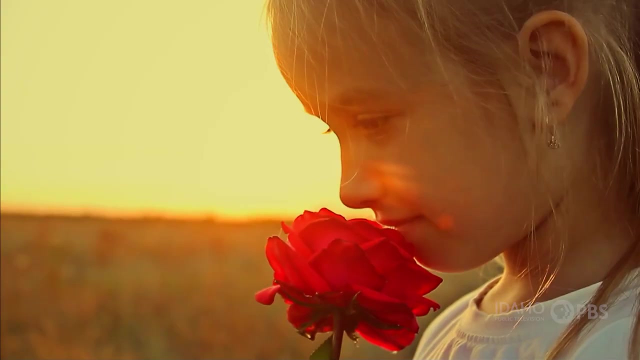 carbon dioxide and other gases in the atmosphere traps heat inside the planet, Like the glass panes keep the warmth of the Sun inside a greenhouse. Carbon dioxide, methane, nitrous oxide and water vapor are all called greenhouse gases. At normal levels, greenhouse gases are good. They keep the planet's temperature. 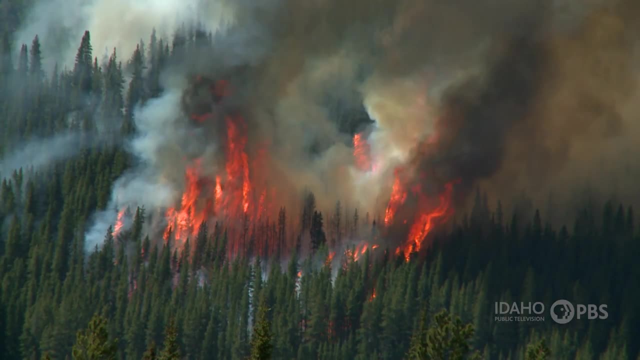 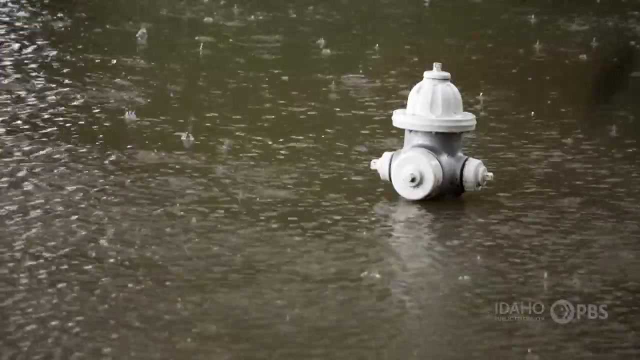 warm enough for us to live. But too much greenhouse gases in the atmosphere means the Earth's temperatures keep going up And as temperatures increase we get melting glaciers, rising sea levels and more extreme weather. It means more plants and animals will go extinct. 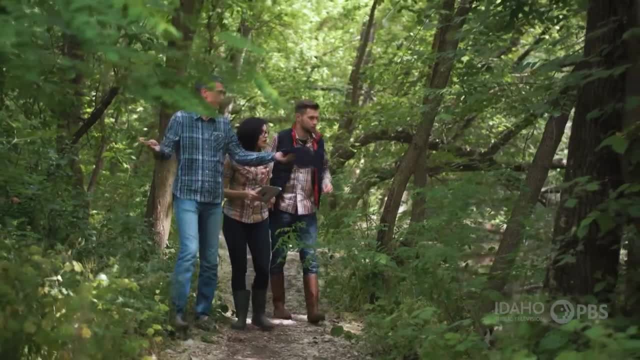 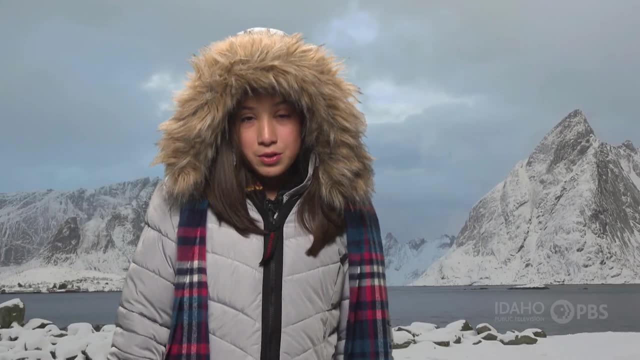 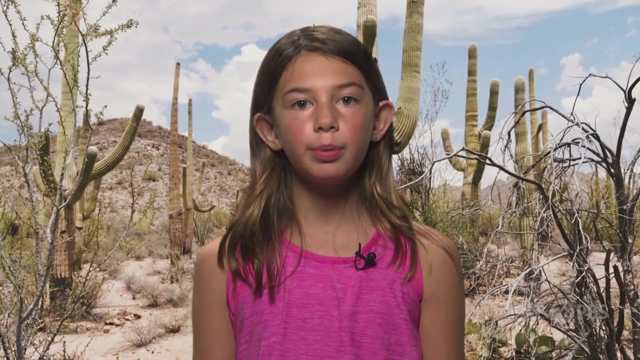 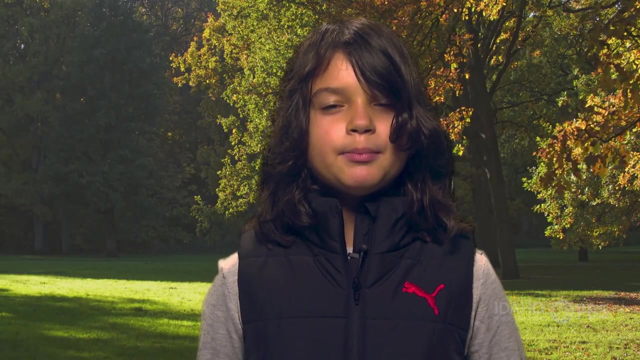 because their habitats and food supplies disappear. Global warming and the resulting climate change impacts everything on Earth, including us. So what can we do? Reduce your carbon footprint: Walk more, drive less. Save electricity. Use energy-efficient light bulbs and off lights, computers and appliances when not in use. plant trees. trees remove carbon from the. 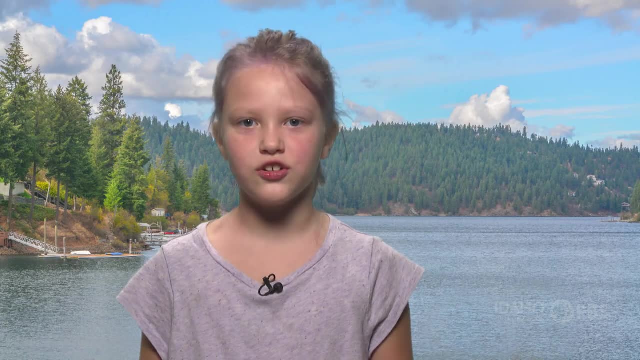 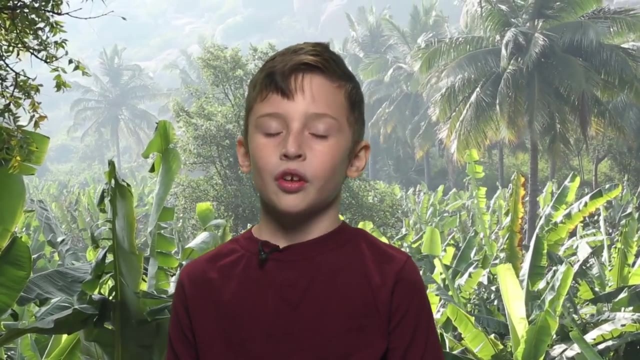 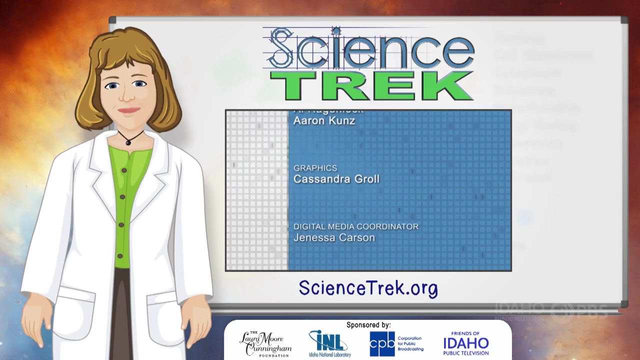 atmosphere. find ways to conserve water and use refillable water bottles and reduce your amount of trash and reuse as much as you can and recycle as much as you can. if you want to learn more, head to the science trek website. you'll find facts, links, games, material for educators and parents. 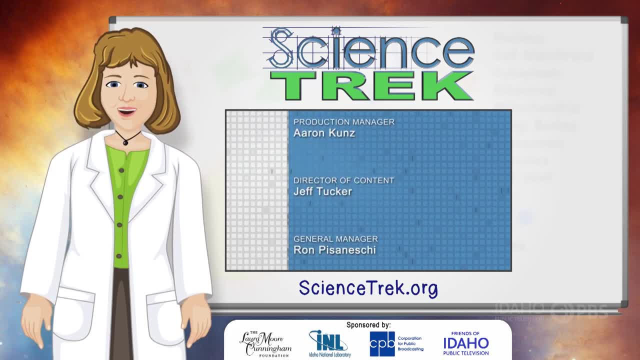 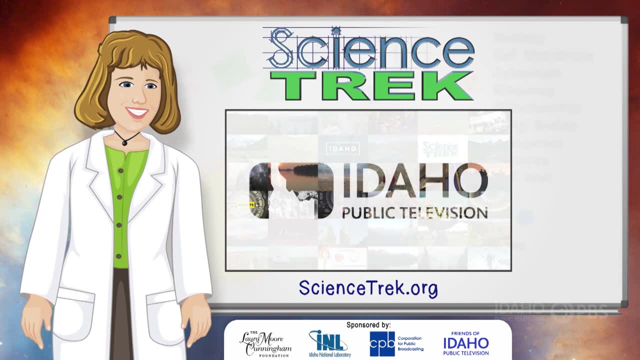 and much more. you'll find it all at sciencetrekorg. 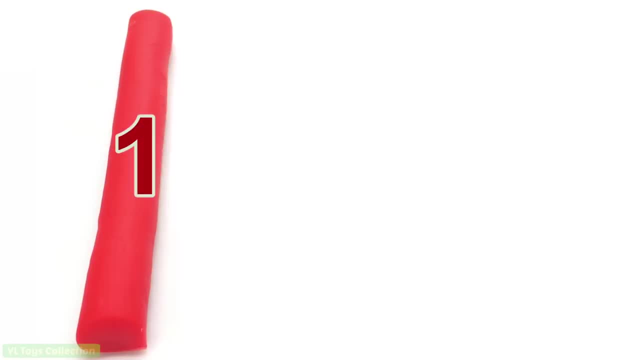 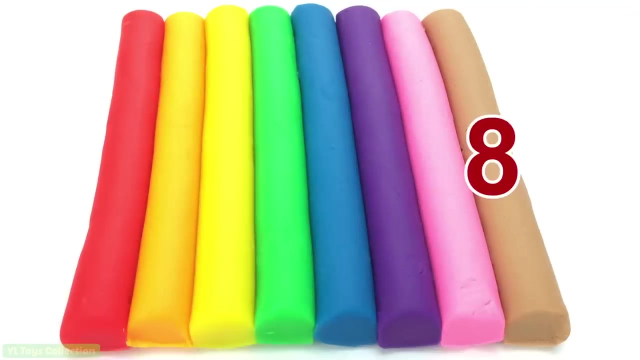 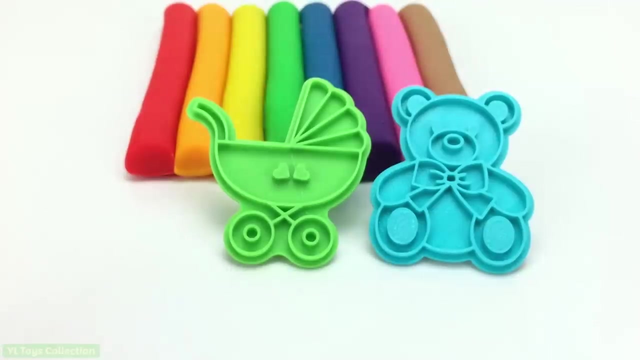 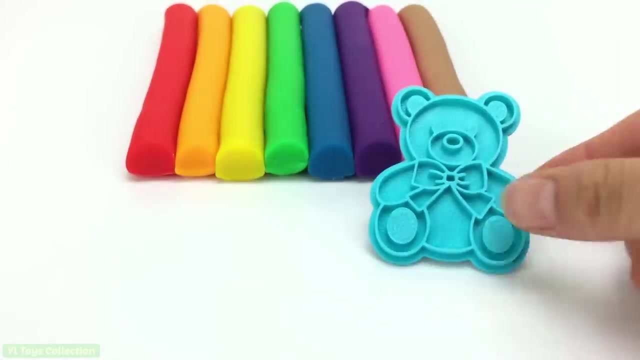 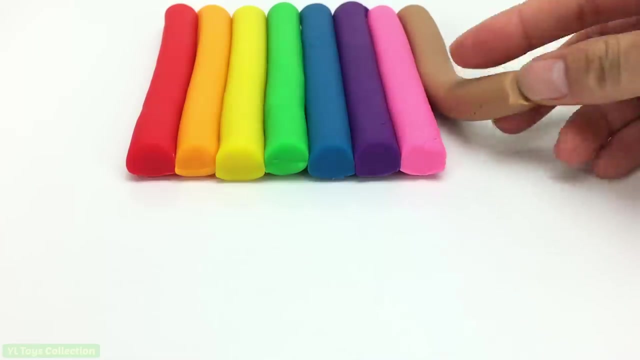 1,, 2,, 3,, 4,, 5,, 6,, 7, 8. 4,, 5,, 6,, 7,, 8, 9, 10,, 11,, 12,, 13,, 14,, 15,, 16,, 17, 18.